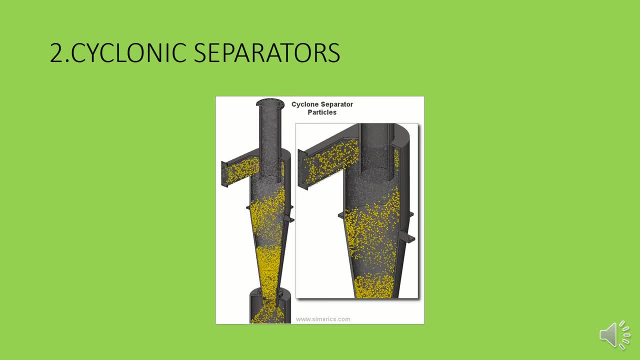 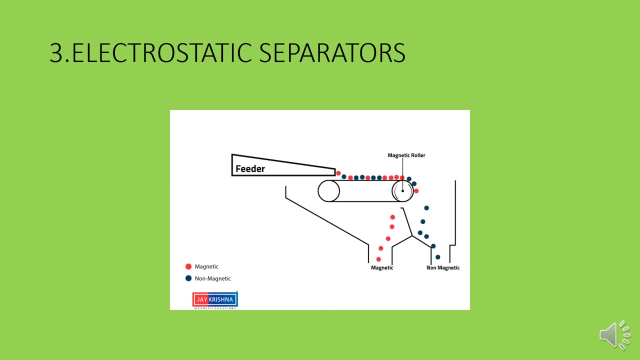 liquid stream without the use of filters through vortex separation. Rotational effects in gravity are used to separate mixtures of solids and liquids. These collect dust particles on the basis of their electrostatic charge. Scrubbers are a diverse group of air pollution devices and there are various types, such as: 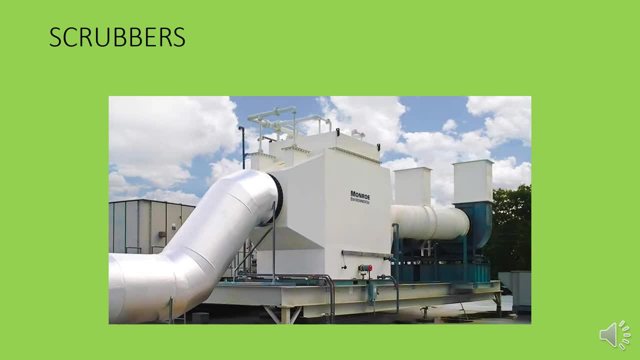 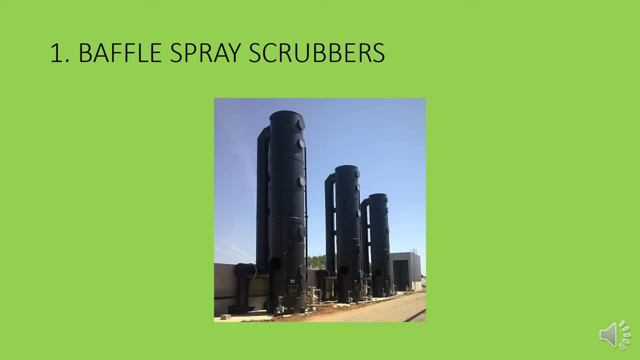 baffle spray, cyclonic spray, mechanically aided spray towers and wet scrubbers. Baffles are added to allow the gas stream to atomize Some liquid as it passes over them. Liquid sprays capture pollutants and also remove collected particles from the baffles. 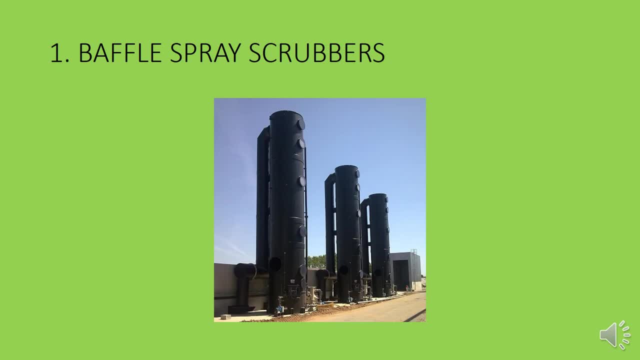 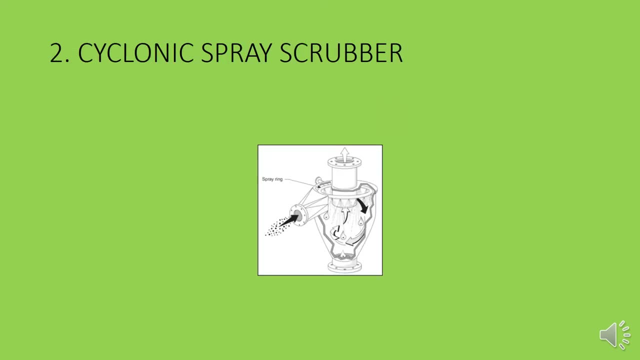 Adding baffles slightly increases the pressure drop of the system, and this is a part of air pollution control technology. Cyclonic spray scrubbers are air pollution control technology. They use the features of both the dry cyclone and the spray chamber to remove pollutants from gas streams. 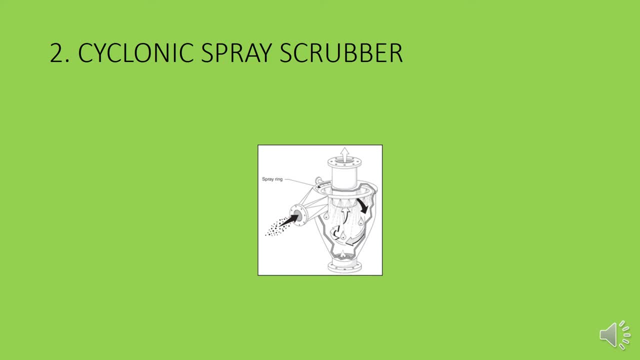 The gas inlet enters the chamber, Swirls through the chamber and exits At some time. liquid is sprayed inside the chamber As the gas swirls around the chamber. pollutants are removed when they impact on liquid droplets that are thrown to the walls and washed back down and out. 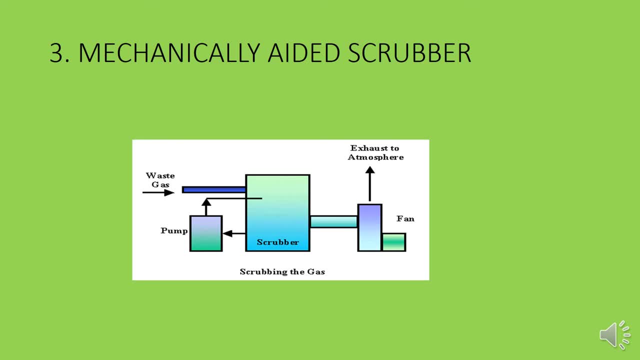 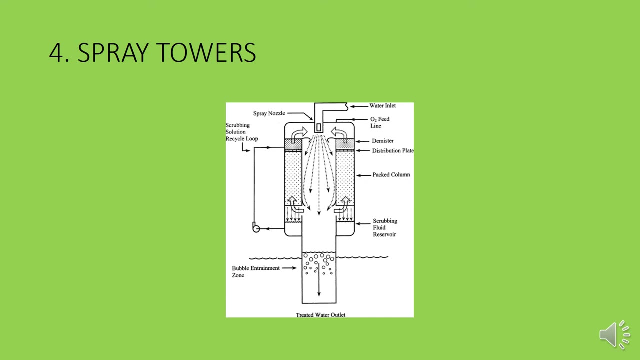 The waste gas enters into the scrubber and the motor that generates electricity rotates the rotor or paddle, which generates water droplets from the exhaust. This system works on counter current flow, because the inlet gas stream usually enters the bottom of the tower and moves upward, while liquid is sprayed downward from one or more. 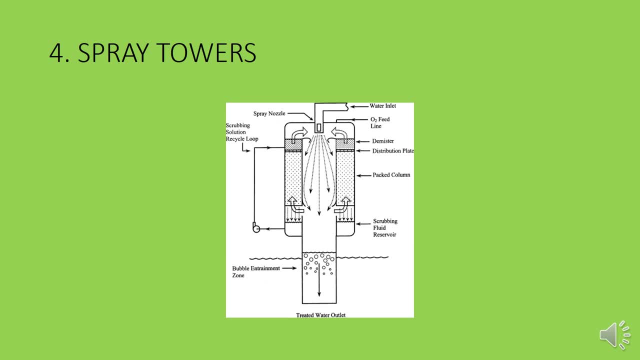 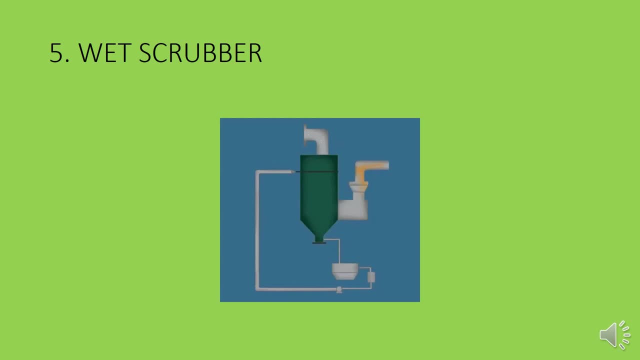 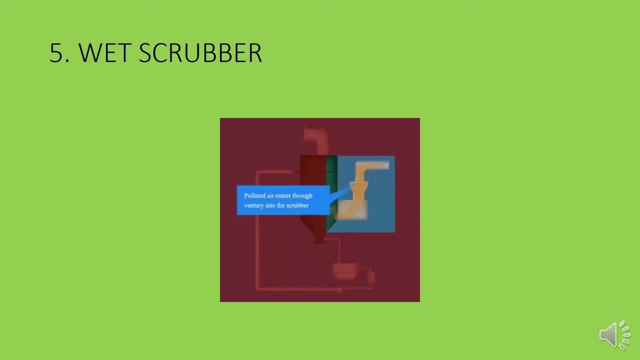 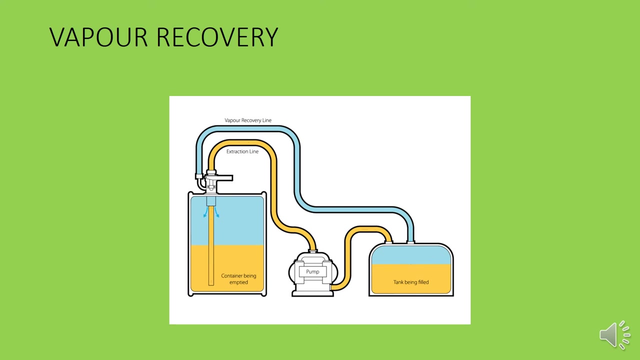 Then the liquid enters the chamber And then the polluted gas stream is brought into contact with scrubbing liquid by forcing it through a pool of liquid. so that's how it removes pollutants. Vapour recovery is the process of recovering the vapours of gasoline and other fuels. so